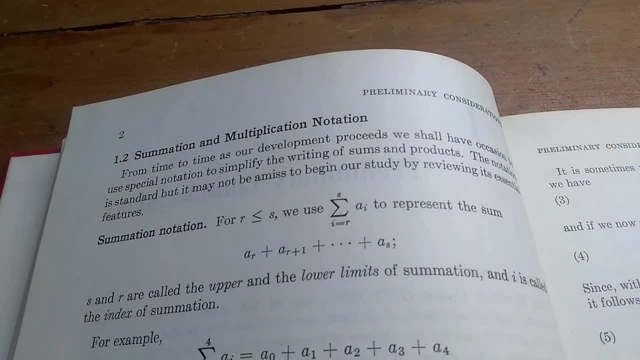 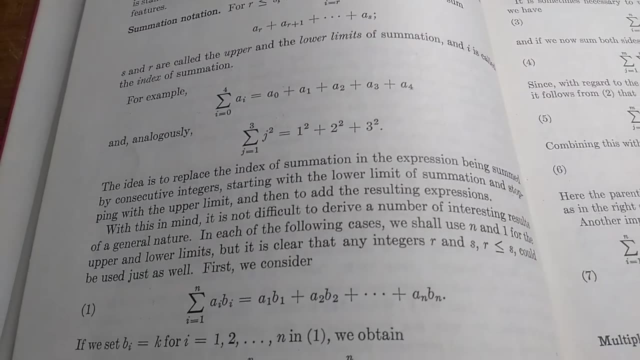 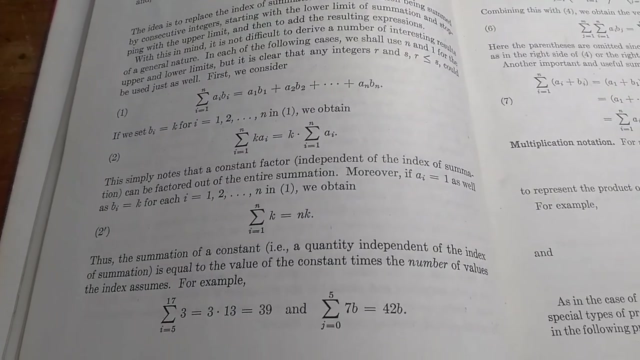 This is a defining element in Rowling's budget. to say, Well, this is a tangible example. In fact it's not, And any time you fill this countinst, you'll totally be able to see how much information is pertained in this example. 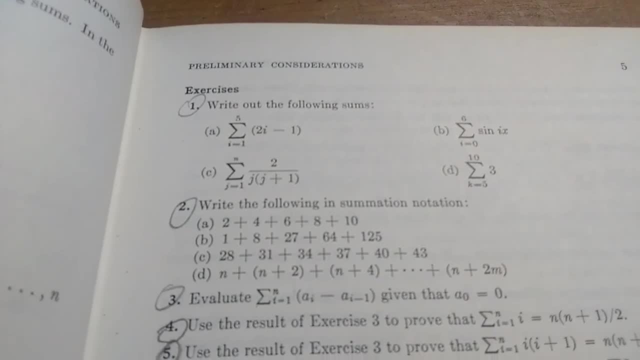 You'll be able. it would be attention Whether your fundamental facts, education, patrol, historyent pugnance or mainly ekedar indicators are在 옥ほ guard predicted NoEL If your module is considered non dość магتен. 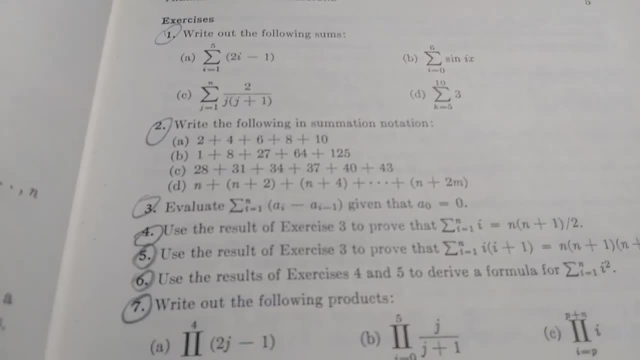 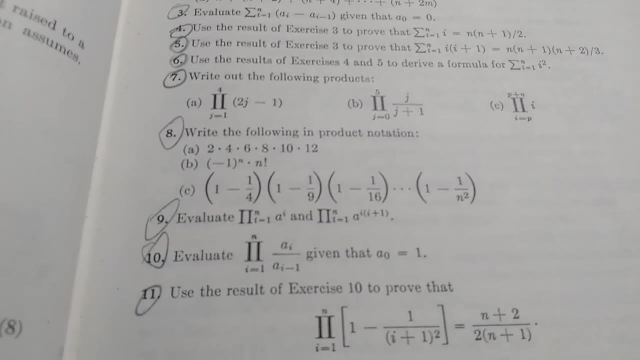 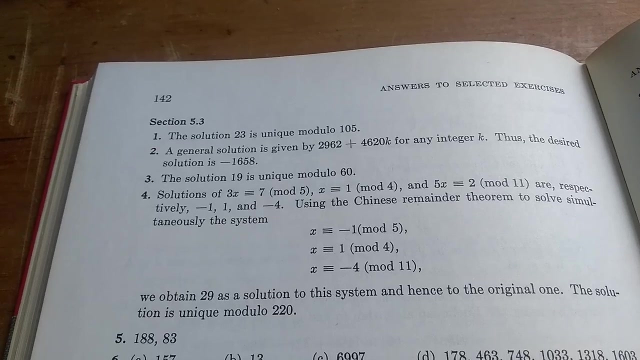 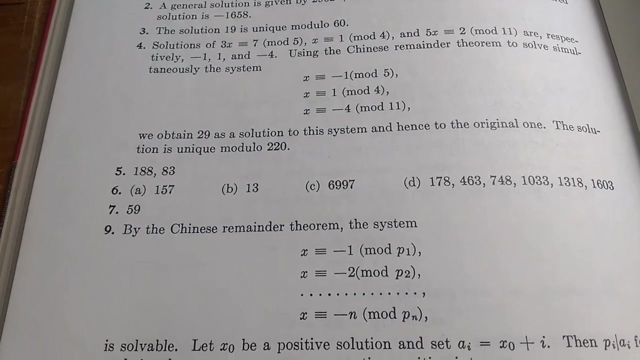 And you know you need some easier problems to make you feel good. So it is a beginner book on number theory. So those are the problems. The author does include solutions to several of the exercises in the back of the book, which makes it a great book for self-study, which again is what I have used this for. 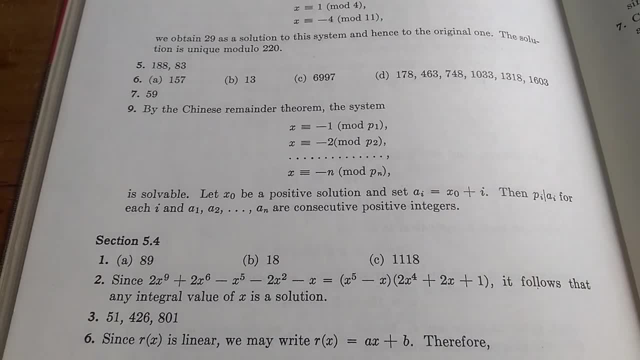 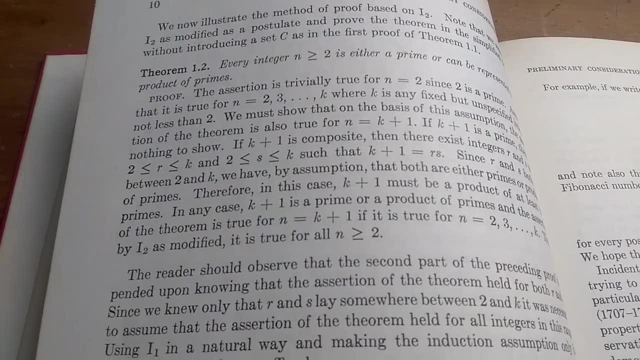 I have never taken a course on number theory. I'm definitely not a number theory expert And again I just want to emphasize that this is actually a really good book to read. I was able to read the book and look at this. 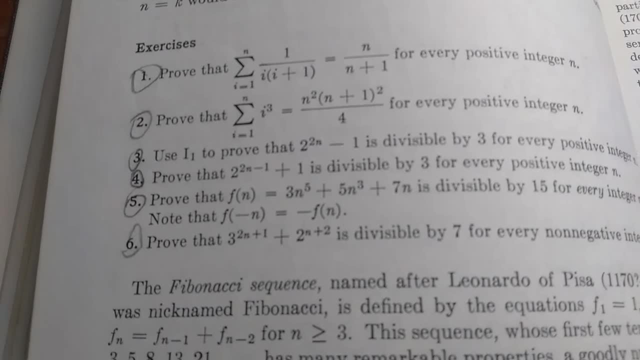 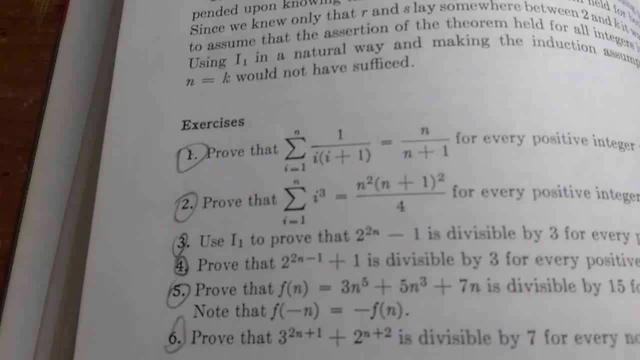 I actually did all of the exercises in this section, So now these are easier exercises. maybe It's just induction problems, But still, you know I did this a long time ago. This is before I even had a math degree. So yeah, it's a really good book.